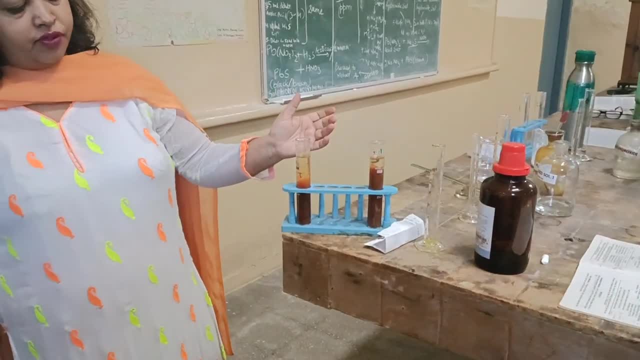 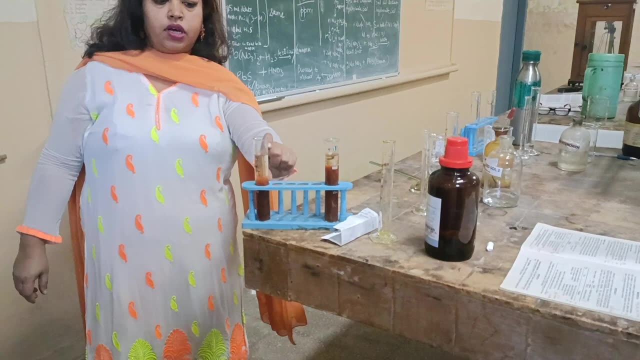 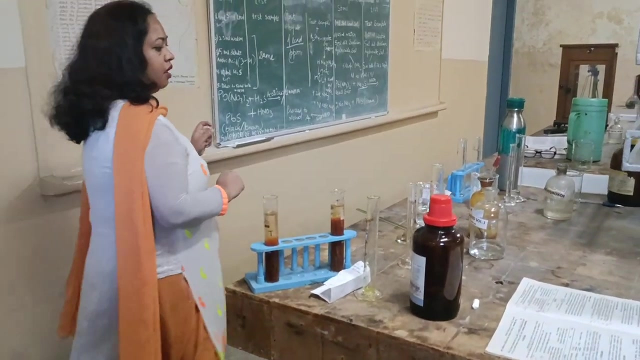 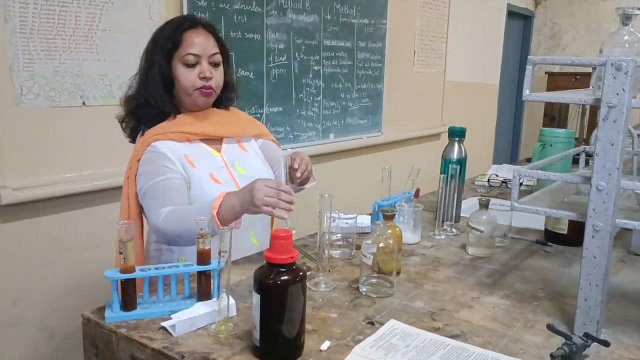 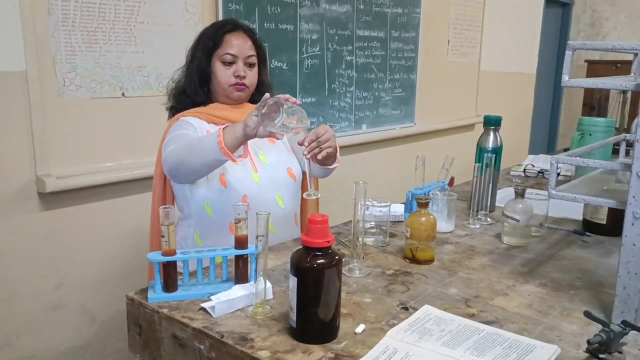 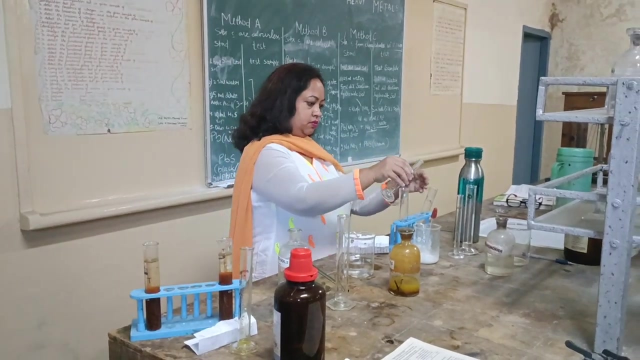 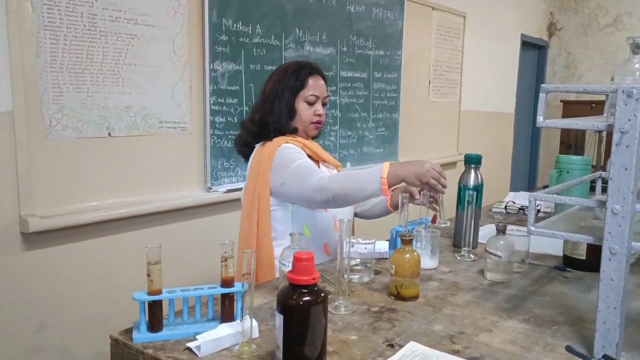 of sodium chloride passes the limit test of heavy metals. We have got beautiful brown colour in the standard and brown colour which is lighter in test. Then for method C will again add 2 ml of lead standard solution. We will add 5 ml of. 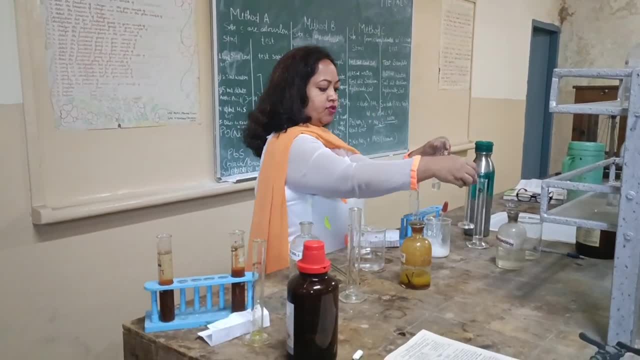 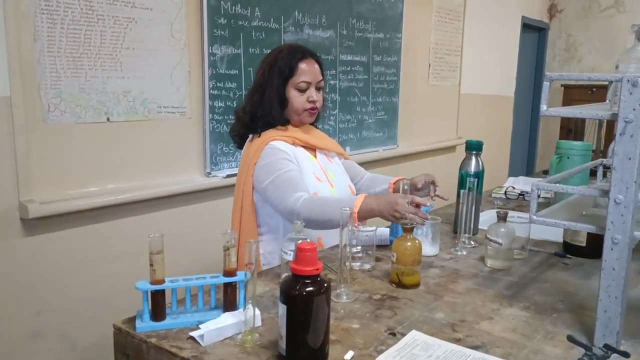 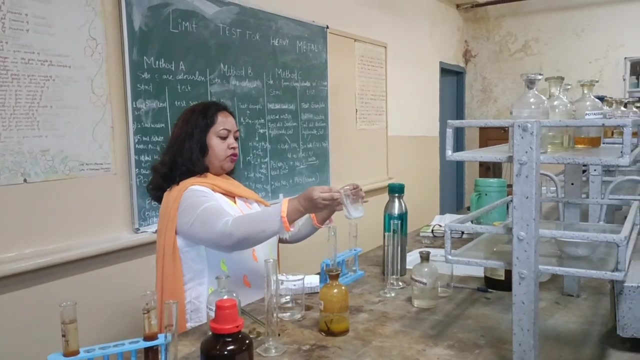 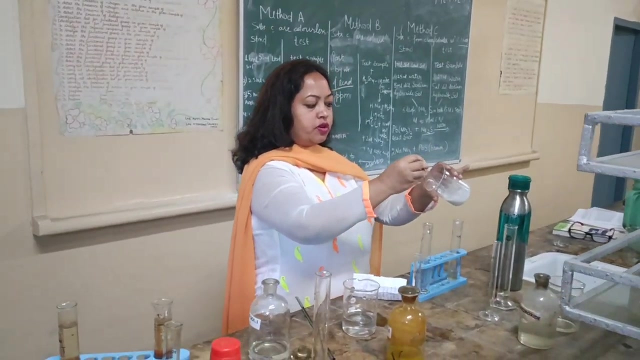 sodium hydroxide in method C, which is giving you the alkaline medium, and five drops of sodium sulfide, which will react with the standard lead solution to give you the sulfides of heavy metal, that is, lead sulfide. so we'll add five drops of